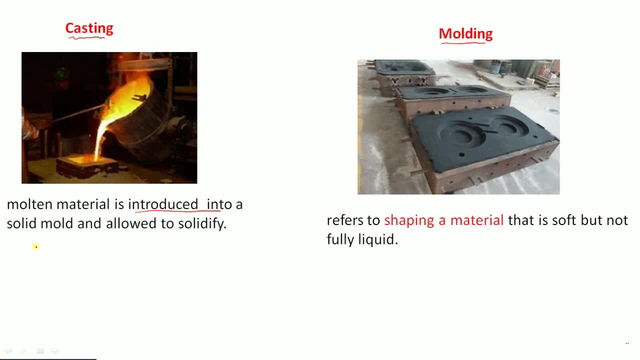 That here molten metal material is introduced into the solid mold and allowed to solidify. So this is called casting, Whereas in molding it refers to shaping a material that is soft but not fully liquid. So we are shaping a material of required shape and size. 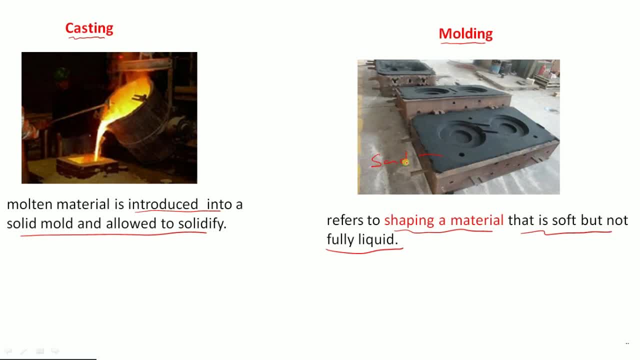 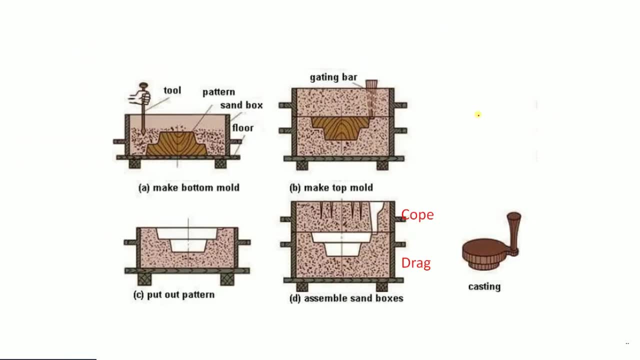 See, here you can see the molding sand And it is shaped like this. It is shaped in such a way that where it can fit a pattern. So, in brief, if we look on the casting initially it will start with the keeping pattern on the mold box. 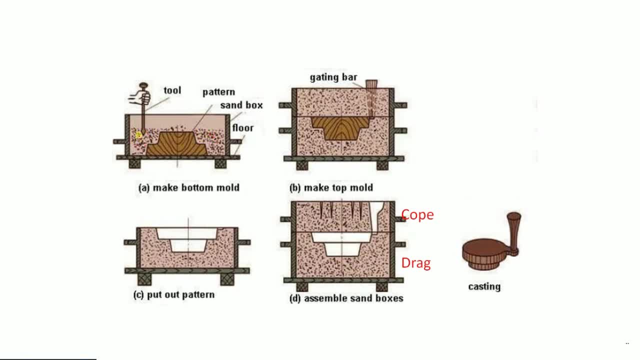 And then we are putting sand all over And, with the help of tool, we are ramming And we are fully covering sand Sand in this mold box. So once it is over, we are putting the upper part of the mold box. This is called probe. 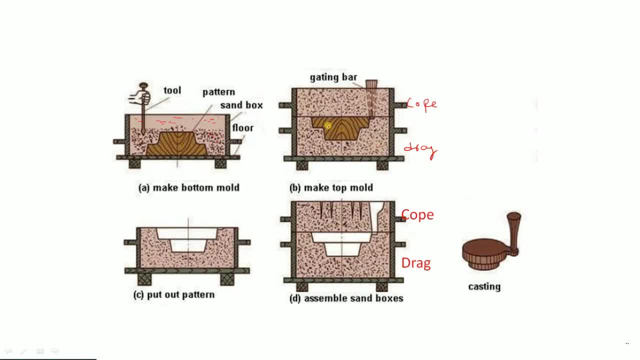 And the lower part is called drag And we have pattern in middle. It may be of wooden, metallic or made up of plastic, And then we are giving the molding And then we are giving the gate and risers. So after this we are again removing the pattern out from here. 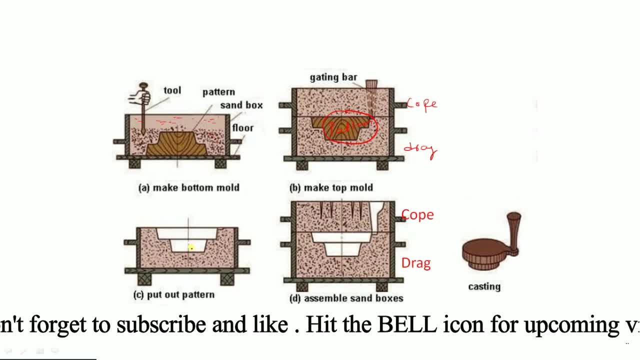 Because if you see the diagram B, there is a pattern In here. pattern is removed, But we obtained the shape of pattern in the sand That is called mold, So we have the shape. So we have the shape of pattern in the mold. 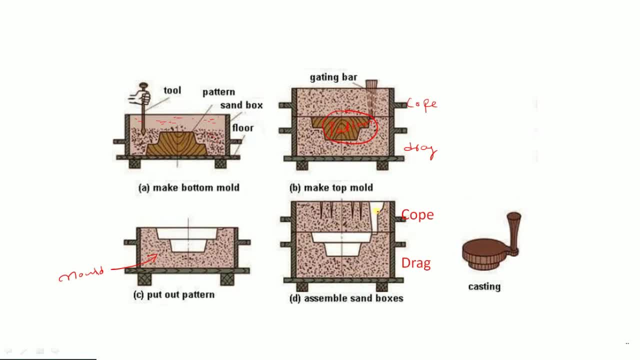 So we are attaching risers and pouring basin and everything, And then we are going to pour the molten metal In the mold cavity. This cavity is called mold cavity. This cavity is formed due to removing the pattern. So once we pour the molten metal, 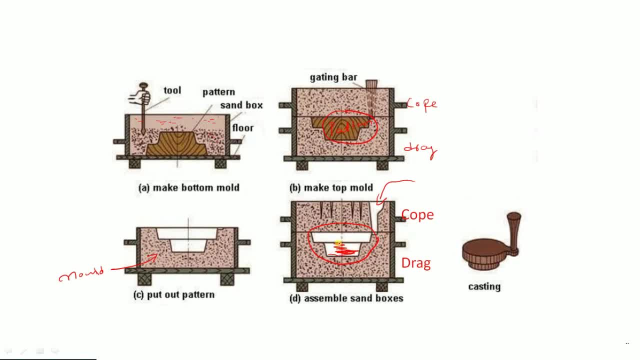 Molten metal will occupy this empty space And it start to solidify. After solidification, we will produce the casting. So, and then we are removing this, risers and gates, And thus we acquire the original diagram That we are required to manufacture. 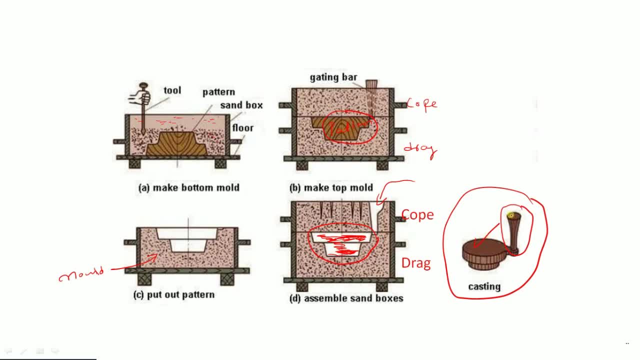 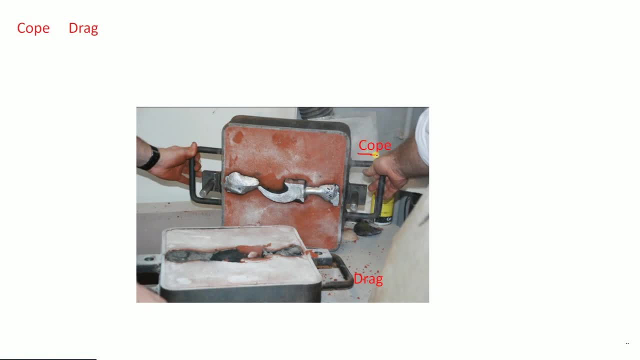 Original shape that we are required to manufacture. So cope and drag. Cope is the upper portion And drag is the lower portion. We can see here. sand is here, That is mold, And when we remove pattern from this space, This hollow space will be called mold cavity. 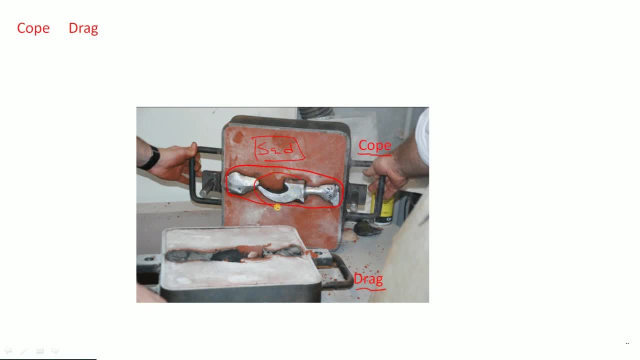 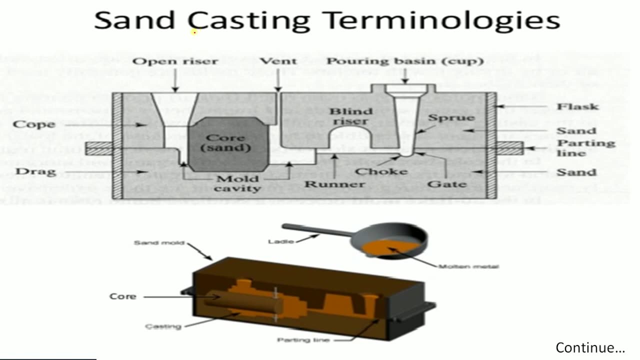 And after solidification we get the casting of this kind. So let's look on the sand casting terminologies. So let's start with the pouring basin. Here we are pouring the molten metal Spur and attachment to the pouring basin Gate from which the molten metal enters. 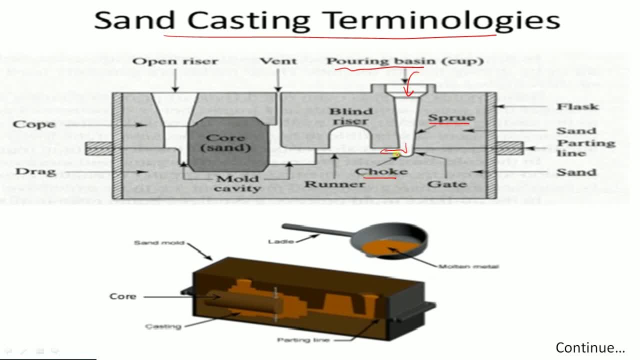 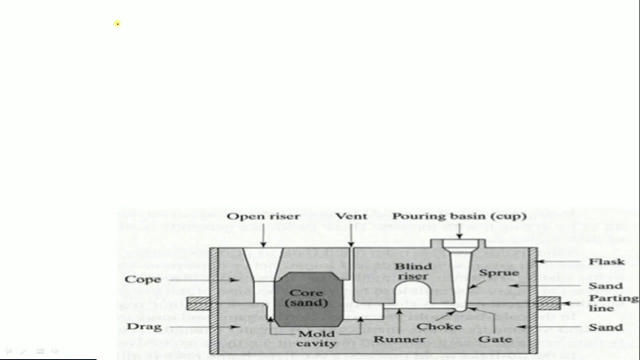 And then choke. There is a curved shape here To arrest the solid particles Dissolved in the molten metal. This portion is called choke Runner, where the molten metal flows. So we have runner. So let's look on the every details. 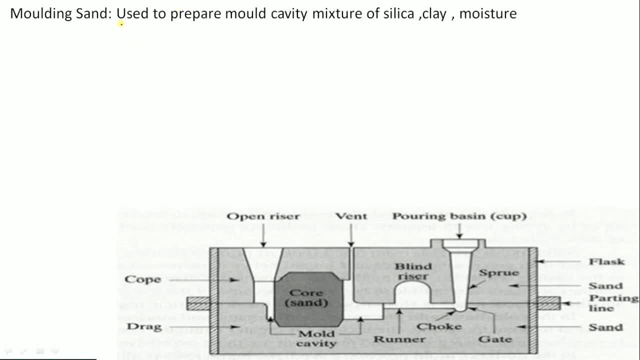 Moulding sand, And moulding sand is used to prepare mould cavity. It is a mixture of silica clay and moisture, So I will explain silica clay in the next slides In detail. Next is core. Core is used to make hollow cavities. 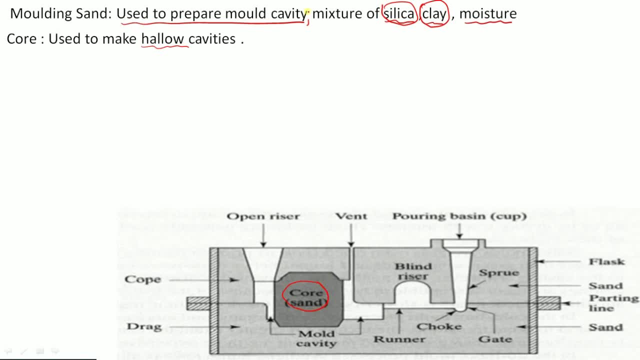 That we can see here Pouring basin, A small funnel shaped cavity at the top Into which molten metal is poured. So we can see the pouring basin. It is a funnel shaped cavity, So where we are going to pour the molten metal. 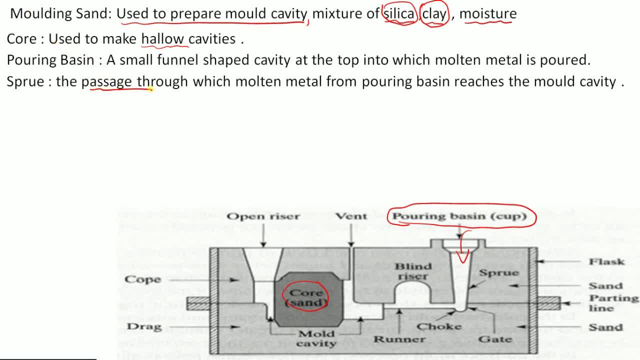 Spur. Spur is the passage through which molten metal from pouring basin reaches the mould cavity. So spur is here. It is an passage through which molten metal from the pouring basin reaches the mould cavity. Runner, the passage in the parting plane. 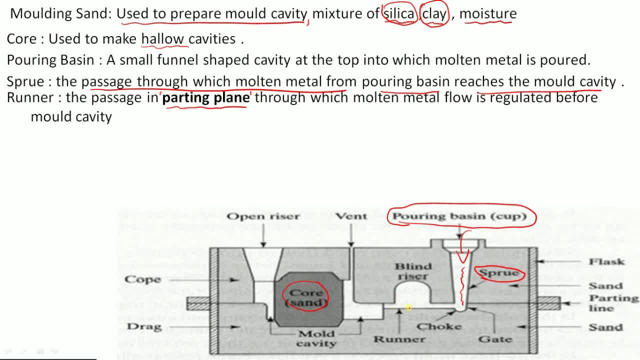 See, we have to remember this thing: The runner used to be in the parting plane. See, the runner is here And we can see the parting line Which divides the cope and drag. We have cope here. We have drag here. 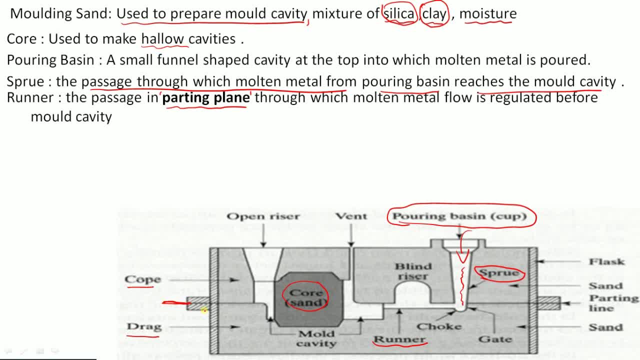 And these two are attached On a certain position And that line is called parting line. In the runner case, The runner is in the parting line always, So the runner is the passage in the parting line Through which molten metal flows. 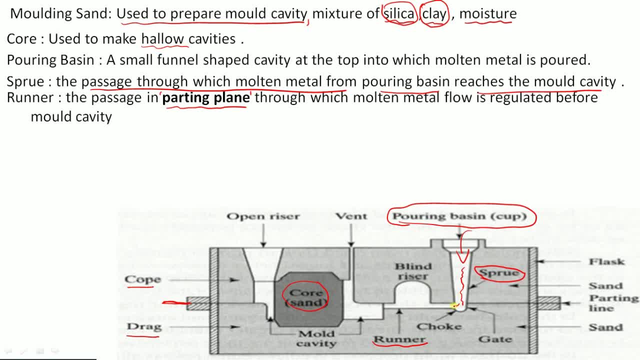 Is regulated before the mould cavity. That means We are regulating the molten metal flow By the runner. So we have gate, The actual entry point through which the molten metal enters the mould cavity In the controlled rate. So this portion is called. 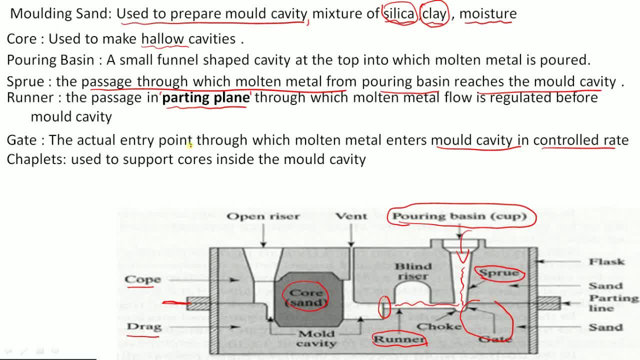 Gate. This is also the gate. It is the entry point Through which the molten metal enters the mold cavity in a controlled rate and then chaplets- chaplets used to support the core inside the mold cavity. so we have pore here. there is something need that will support the pore.